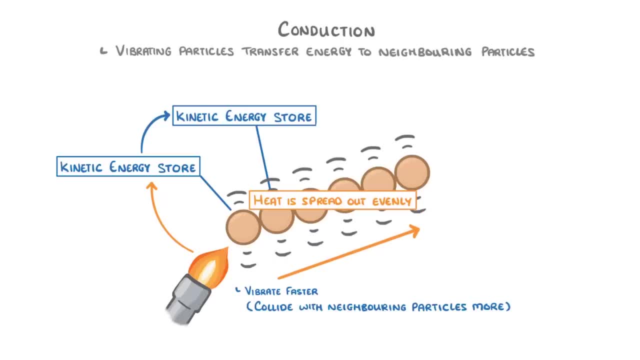 Now, the reason that conduction occurs mainly in solids is because the particles in a solid are held together really closely, which means that there's lots of collisions that pass on the energy, Whereas in liquids and gases the particles are all further apart, and so 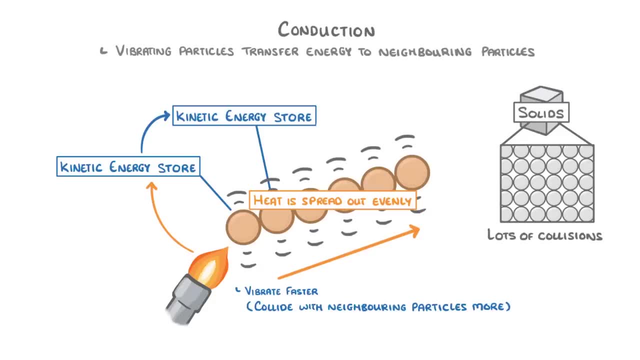 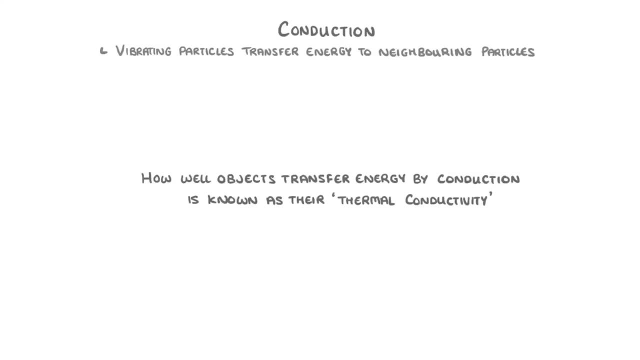 they don't collide as much. Exactly how well objects transfer energy by conduction is known as their thermal conductivity. Metals have a high thermal conductivity and transfer heat energy rapidly, Whereas plastics have a low thermal conductivity, which is why we use them as insulators And pretty. 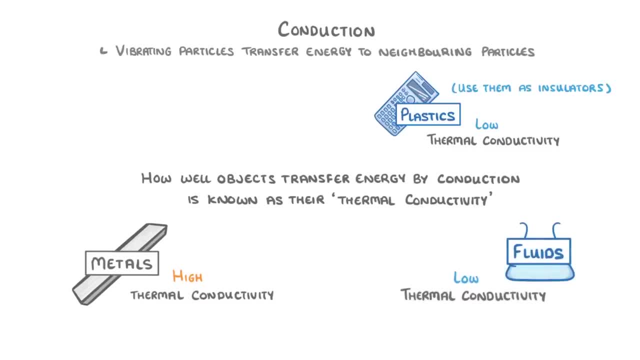 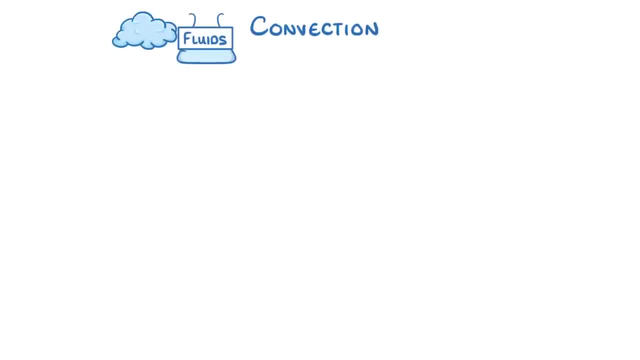 much all fluids have a low thermal conductivity. Convection, on the other hand, occurs mainly in fluids and remember, fluids can refer to anything that can flow, so both liquids and gases. Convection, on the other hand, occurs mainly in fluids and remember, fluids can refer to. 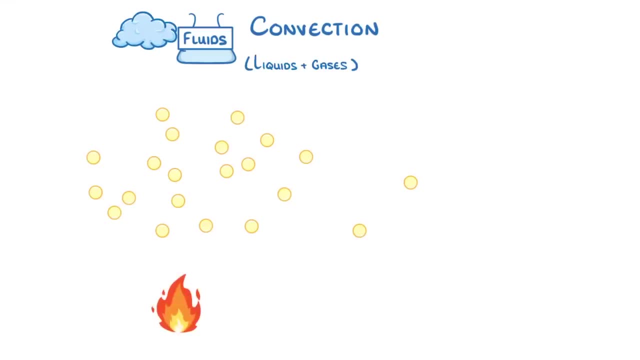 anything that can flow, so both fluids and gases. Because the particles in fluids aren't fixed. once they're heated and they gain kinetic energy, they all move around faster By the process of random diffusion. these will cause these more energetic particles to move away from the warmer region towards the cooler. 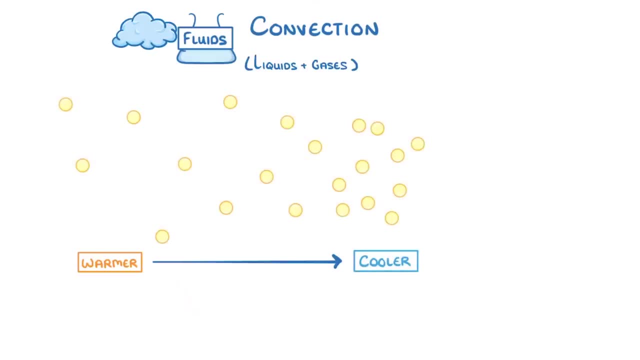 region And overall this means that the higher energy particles in the warmer region are a lot more spread out than those in the cooler region. So, effectively, the fluid in the warmer region actually expands as it heats up, and so it becomes less dense than the cooler fluid. 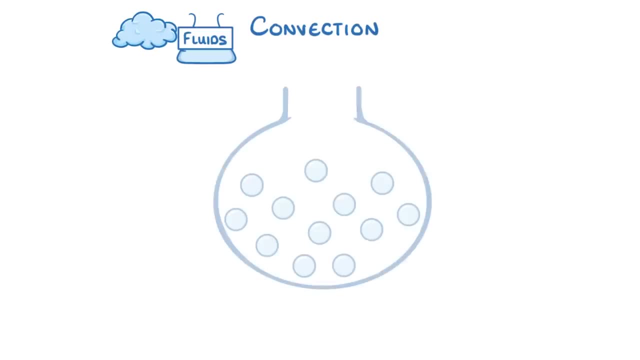 To understand how this works in real life, let's imagine that we had a container of fluid, so that could be either liquid or gas. As we heat the container, the following things would happen. First, the particles near the heat source would gain kinetic energy and 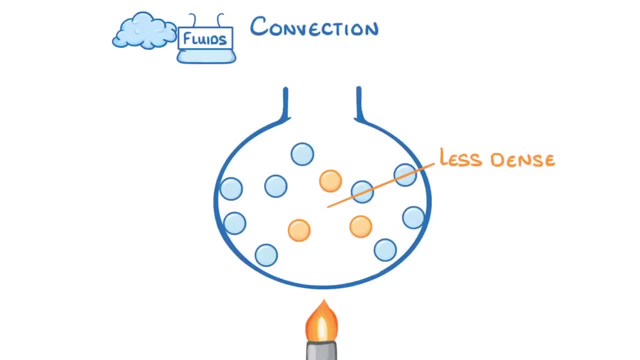 spread out, becoming less dense. Because they're less dense, they're not as dense as the other particles in the cooler region. And because they're less dense, they're not as dense as the other particles in the cooler region. And because they're less dense, they're not. 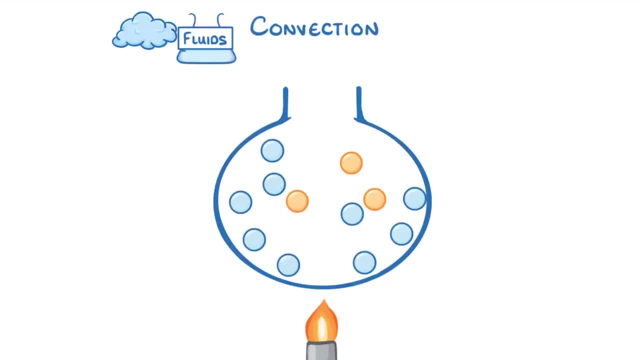 as dense as the other particles in the cooler region. These particles rise above the colder, less dense particles above them, And at the same time, these cooler particles sink down and take their place. Whilst this is happening, though, the hot particles would lose their